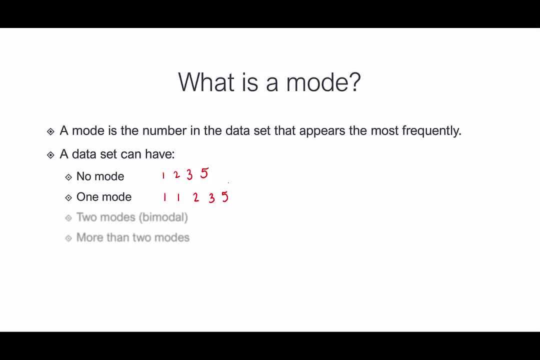 other value in the data set, It appears twice. The 2,, 3, and 5 each appear once. So this would have one mode, and that one mode is coincidentally 1.. So the one mode in this would be 1.. We. 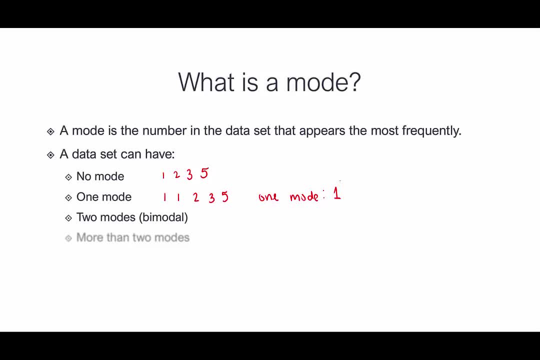 could also have a data set with two modes. We call that bimodal, bimodal. A bimodal data set is a prefix that means 2.. So a bimodal data set means that we see two numbers that appear more than any other number. So what if we had 1, 1, 1, 2, 2, 3.. 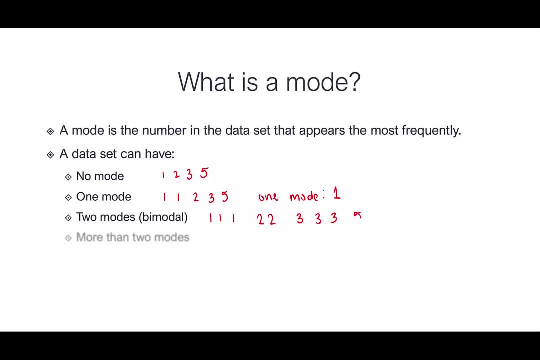 I don't know why I'm bunching them all together: 3, 5.. In this case, we have two modes: 1 is a mode and 3 is a mode. They both appear 3 times, which is more than any of the other. numbers, which in this case is 2 and 5.. 1 is a mode and 3 is a mode. They both appear 3 times, which is more than any of the other numbers, which in this case, is 2 and 5.. 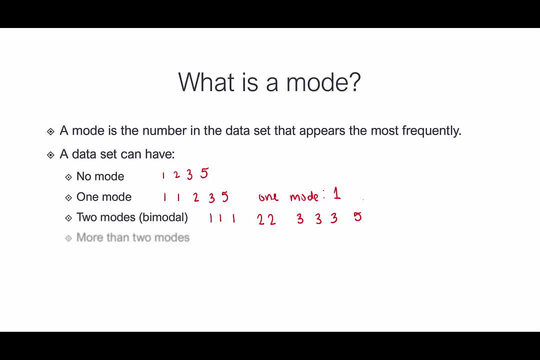 1 is a mode and 3 is a mode. They both appear 3 times, which is more than any of the other numbers, which in this case is 2 and 5.. So because 1 and 3 appear more than any other number, so 2 does appear more than once. 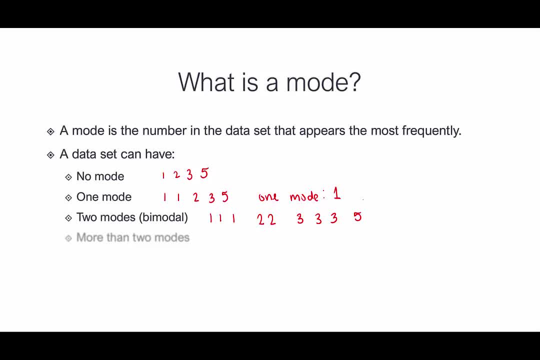 but it only appears twice. it's not as big as 3,, so we have two modes And the two modes are the ones that repeat 3 times. We would have 1 and 3.. We can also have a data set with more than two modes. So again, in order for one of the 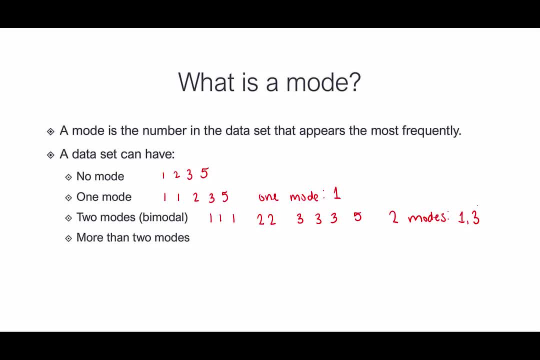 values. to be a mode, it has to appear more frequently than all of the other numbers or equal to. It's like greater than or equal to. So if we have more than two modes, we might have 1, 1,, 1,, 2, 2, 2, 3,, 3,, 3,, 5,, 7,, 8,, 9,. 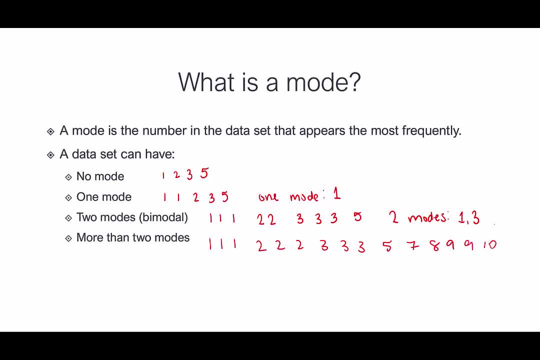 9, and 10.. In this case, this data set would have three modes: right, Because 1 appears three times, 2 appears three times and 3 appears three times 5,, 7,, 8, and 10 each. 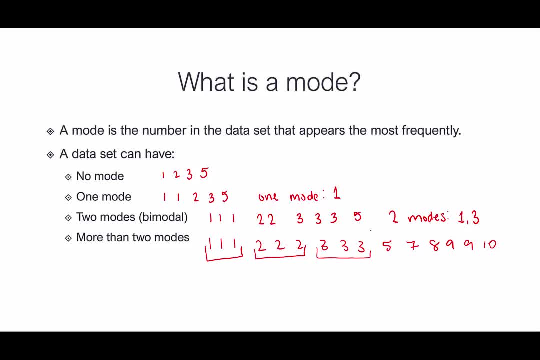 appear once And 9 appears twice. So the numbers that appear more frequently than all the rest are 1,, 2, and 3.. So this one has three modes, and the three modes are 1,, 2, and 3.. 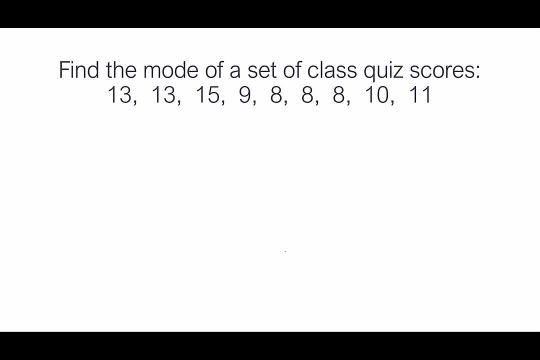 Okay, let's look at a few more examples. I always encourage you, now that we've gone over the definition, pause the video and see how you do on your own, and then you can check back with me. We want to find the mode of a set of class quiz scores, The first thing I want to do 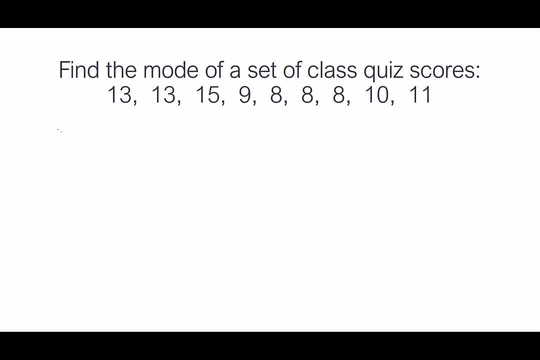 is. put them in order from least to greatest. So when I go from least to greatest, I'm going to start with the 8s: 8,, 8,, 8.. Then I have 9,, 10,, 11,, 9,, 10,, 11.. Then I have 2 13s and 1, 15.. So, as I was writing these, did you pick? 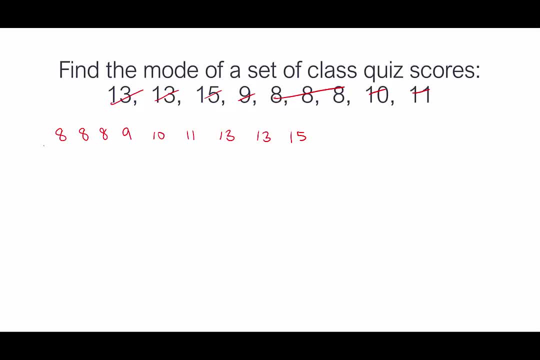 up on the mode Which one appears more than all the rest. That would be the 8.. The 8 appears three times, Whereas the 9,, 10,, 11, and 15 each appear once. 13 appears twice, but 8 is more frequently. 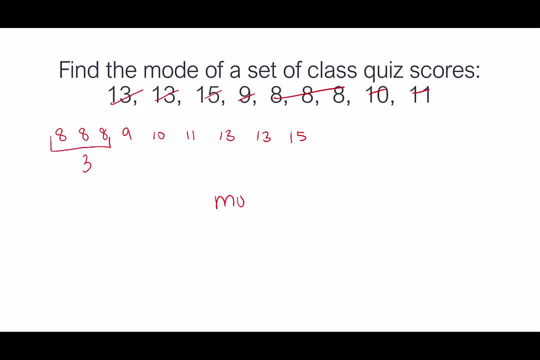 seen than any other quiz score. So we would say the mode quiz score is 8.. It's the data value. It's not the number of times it appears. That's called the frequency. It's the value that's in the data set. So 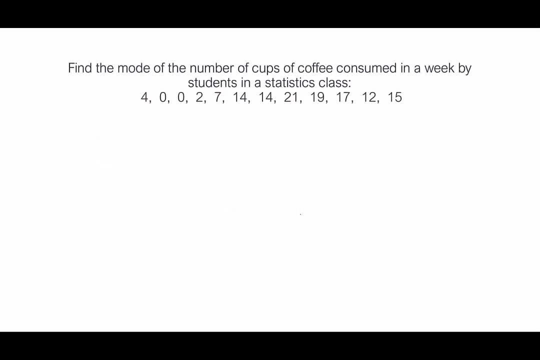 the mode is 8.. How about? in this example? we want to find the mode of the number of cups of coffee consumed in a week by students in a statistics class. I'm going to put them in order first. So I have 0,, 0,, 2,, 4.. Like they're all kind of bunched together. There's not in the right. 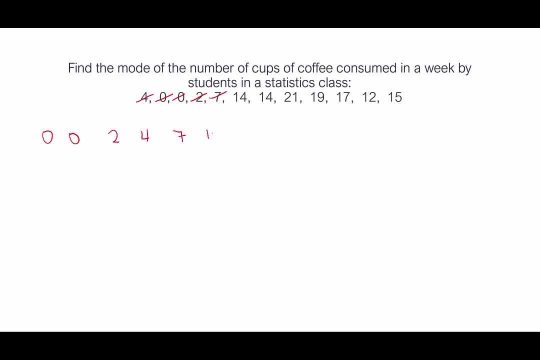 order. Then we have 7,, 12,, 14,, 14,, 15,, 17,, 19, and 21.. So, in this case, have you identified the mode or modes? Say it with me now. There are two modes. I see 0 appears twice and 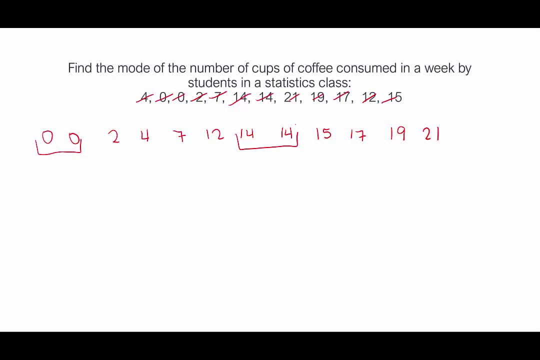 I see 14 appears twice. So 0 and 14 have a frequency of 2. Making this a bimodal data set. So we say bimodal and the two modes in this data set are 0 and 14.. And again, so we don't go with the frequency, We go with the values in the 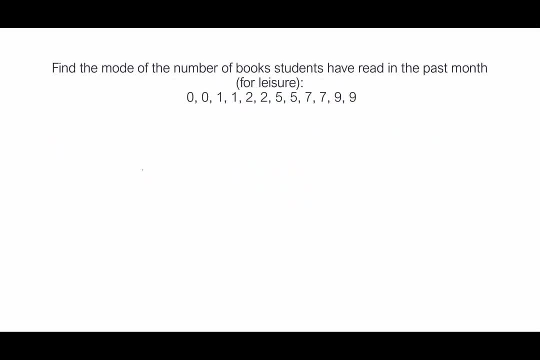 data set 0 and 14.. In our last example, we want to find the mode of the number of books students have read in the past month And look at that. They're nice and in order for me. Okay, so I see the.